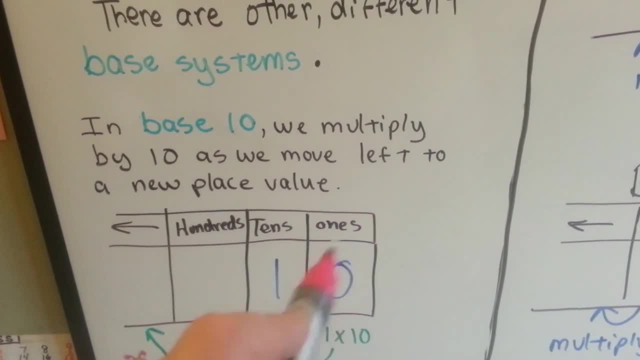 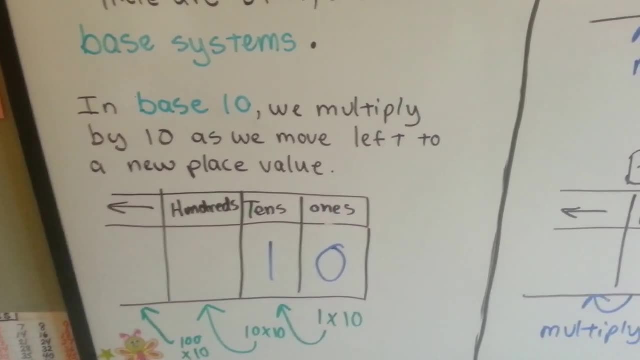 we put a line here and a 0 here to represent nothing. Every time we want to move to the next place value, we multiply by 10.. Okay, well, what's the big deal? Why am I showing you this? This is why. 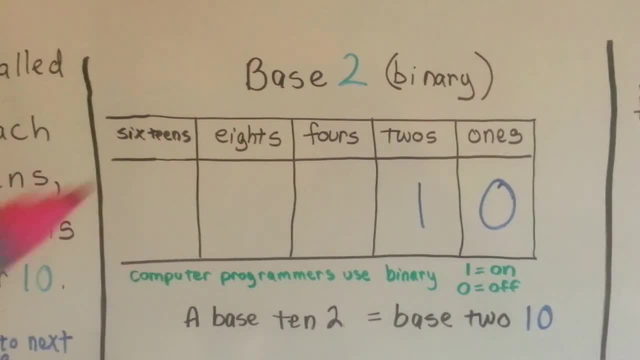 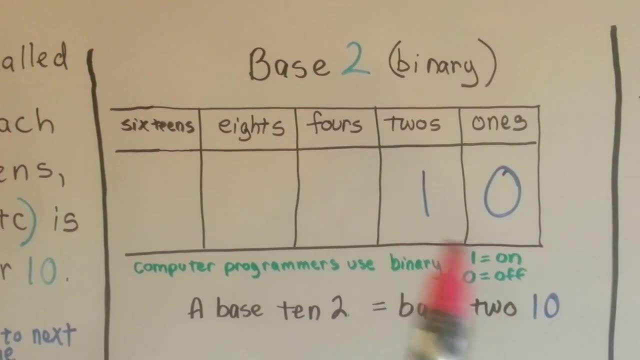 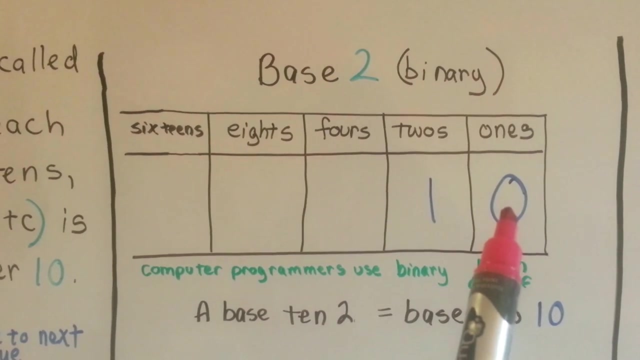 There are other base number systems. Base 2 is called binary and the way it works is: every time you move to an X place value, you multiply by 2.. Each time you're multiplying by 2, you have a 1's place value, and they don't have a 10's place value here, they have a. 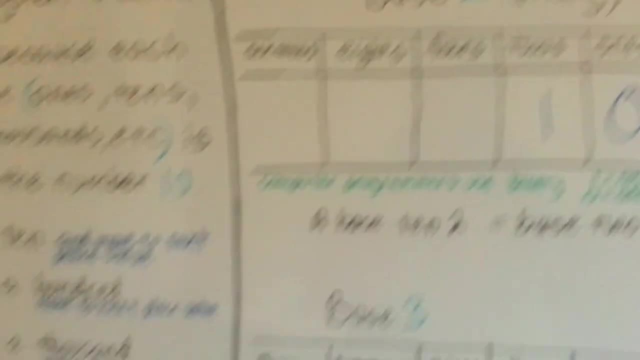 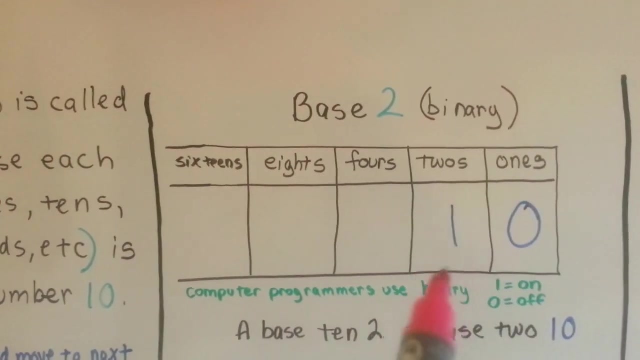 2's place value because it's base 2.. See, In base 10 we have a 1's and then a 10's place value. In base 2 we have a 1's and a 2's. The next place value would be 2 times 2. 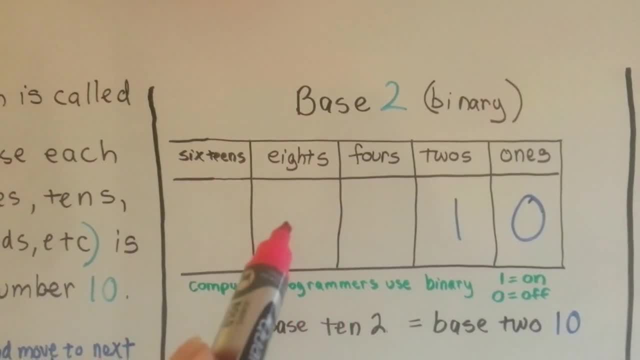 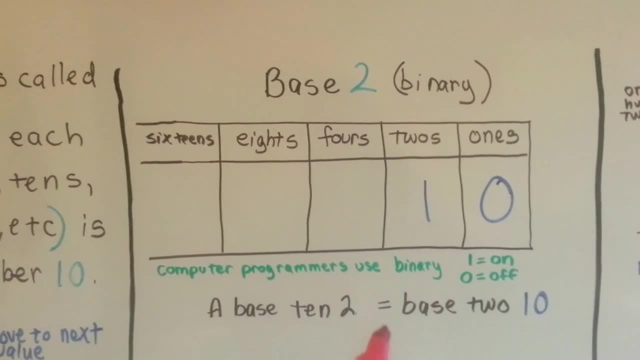 that's 4.. 4 times 2, that's 8.. 8 times 2, that's 16.. So if we wanted to write the number 2 in base 2, in binary, we would write a 1 and a 0. 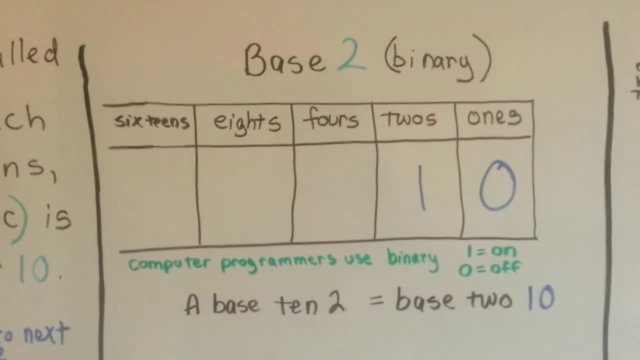 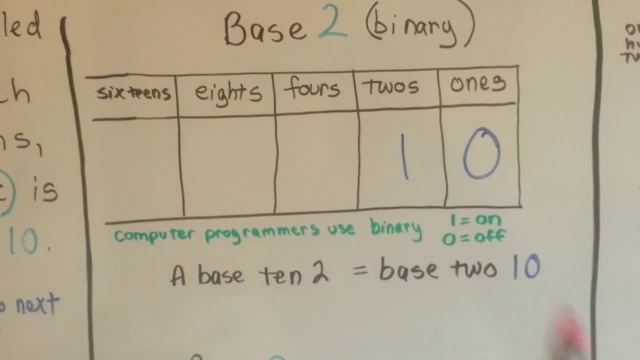 and that would mean a 2 and no 1's. Then we would have a base 10 too, like this, see, But in base 2 in binary it's written as a 1 and a 0, because it represents a 2. 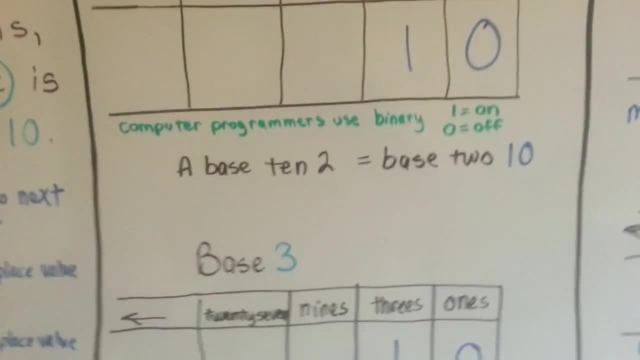 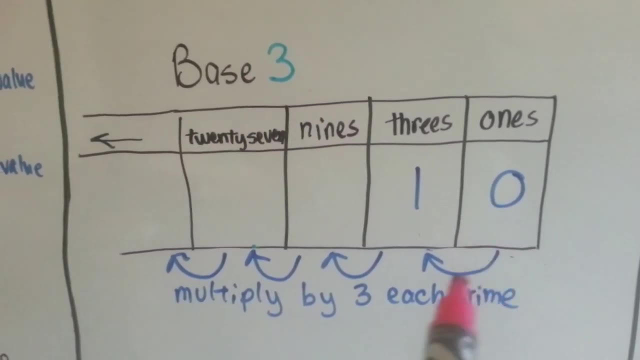 and 0- 1's. Okay, I'm going to blow your mind. We're going to keep on going. In base 3, we multiply by 3 each time You have a 1's column and, because it's base 3, the very next column is 3's. 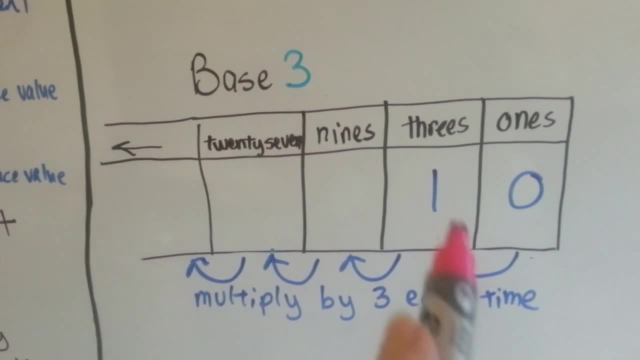 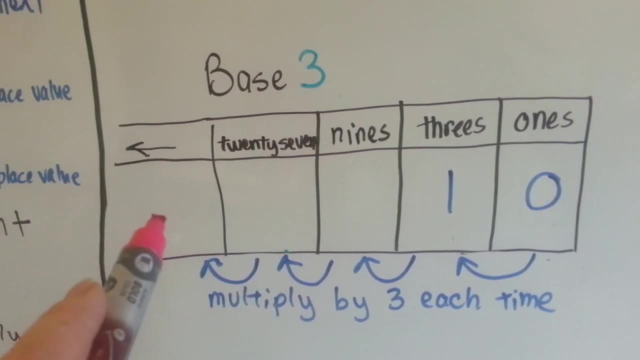 And every time you move to a new place value in base 3 you multiply by 3.. So 3 times 3 is 9, 9 times 3 is 27, and then you would do 27 times 3 for the next one. 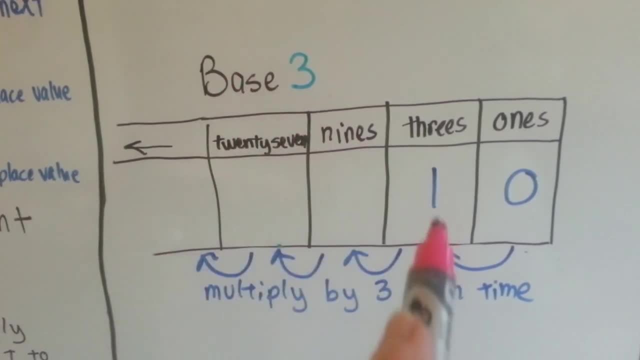 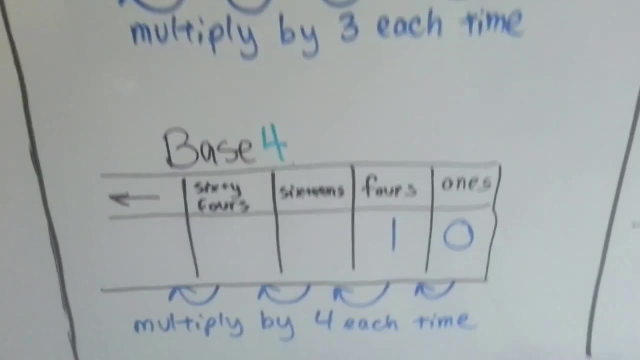 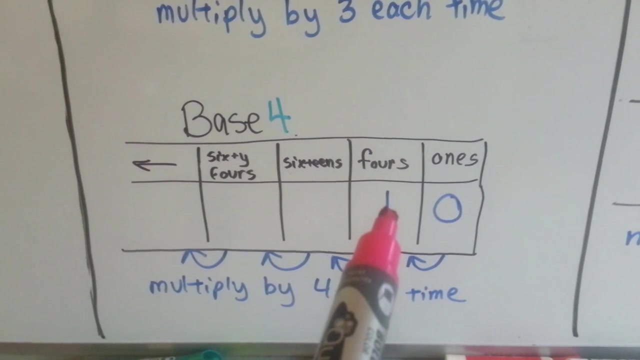 See, To write the number 3 in base 3, you would write a 1 and a 0, because it represents 1, 3 and 0 1's. Okay, in base 4, you multiply by 4's for each place value. We have a ones column and then the very next column is: 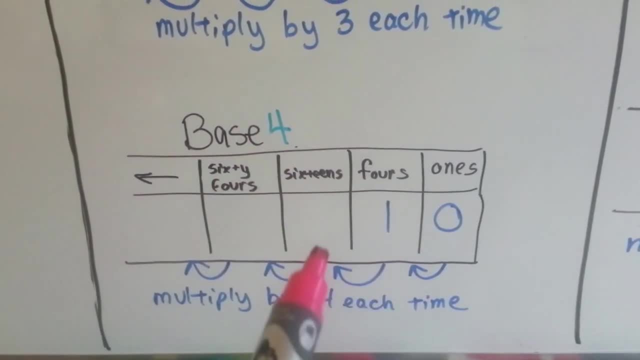 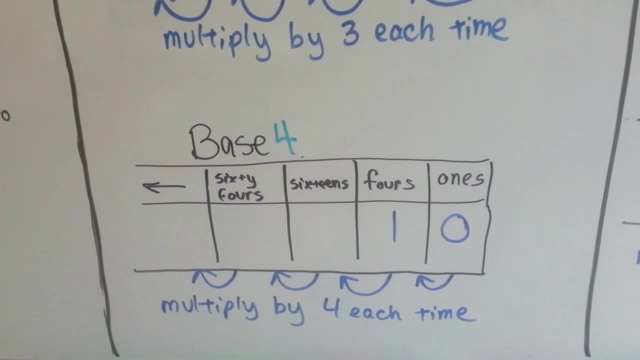 4's because we're in base 4.. 4 times 4 is 16.. 16 times 4 is 64. And those are place values. See, We multiply by 4 each time we move to the left, just like in the base 10. 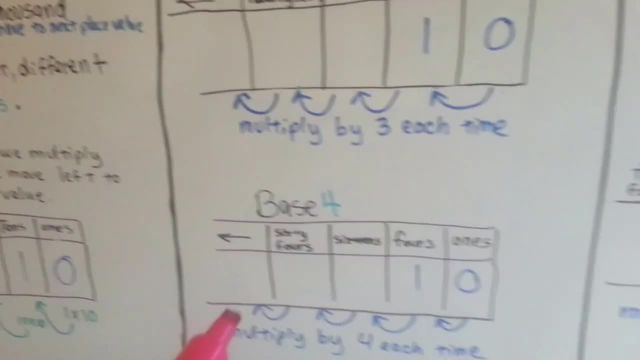 we multiply by 10. See, We multiply by 4 each time we move to the left, just like in the base 10, we multiply by 10.. 10. See, Whatever the base is is how much you multiply to the next column In base 5,. 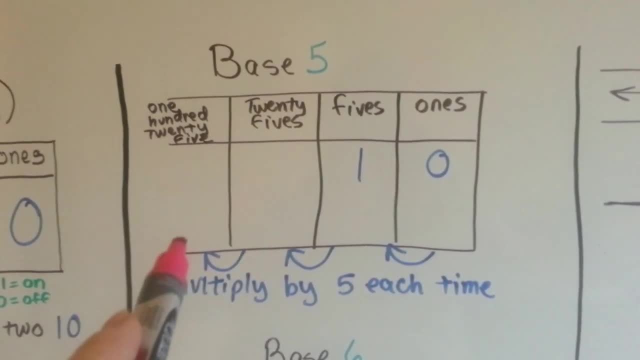 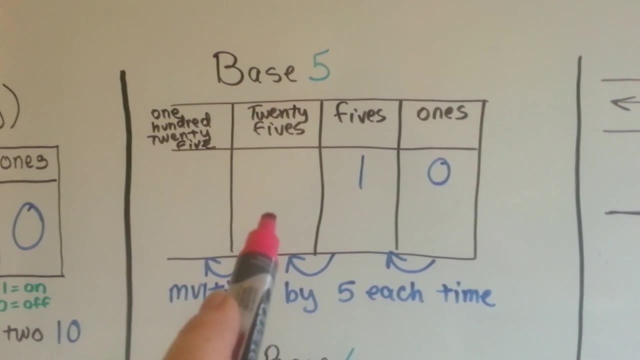 it's the same thing. We multiply by 5 every time we move to a next left place value, You have your 1s. 1 times 5 is 5.. 5 times 5 is 25.. 25 times 5 is 125.. So those are your place. 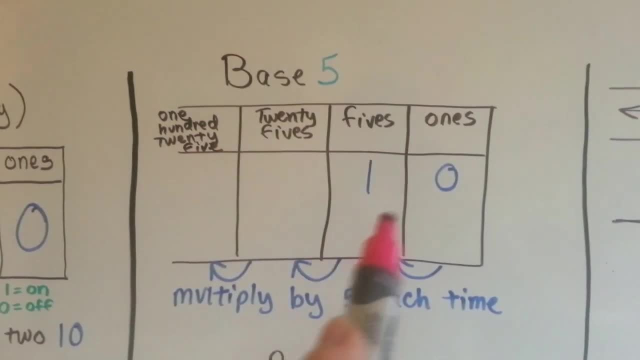 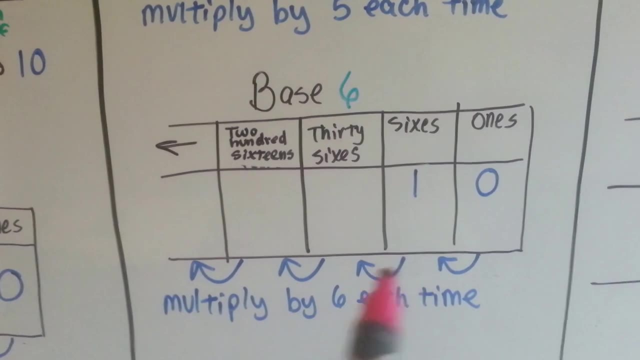 values. To write the number 5,, you would write a 1 and a 0 to represent one 5 and no 1s In base 6, it's the same thing. We're multiplying by 6. You have your 1s and your 6s And the. 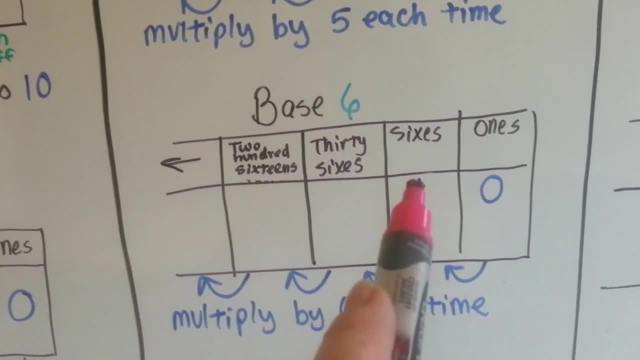 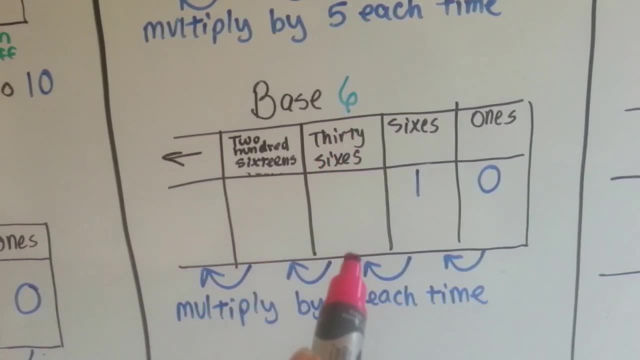 minute. you see, the second column is 6, you know it's base 6.. See, That's how you know what base you're dealing with. 6 times 6 is 36.. So this is the 36s column, 36 times 6. 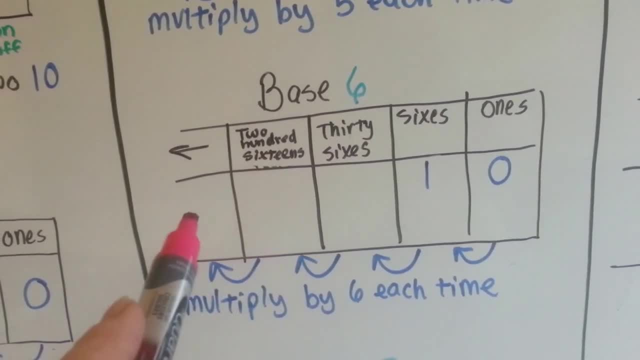 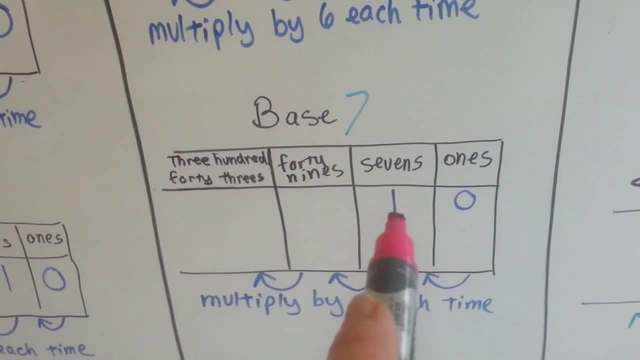 is 216.. So this is the 216s column. And then you multiply by 6. again Same with base 7.. You multiply by 7 every time you move over. Here's your 1s column, your 7s column, So. 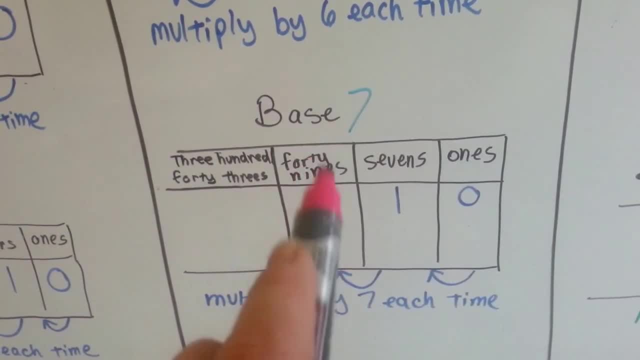 we know that base 6 is 6.. And then you multiply by 7.. You multiply by 7 every time you move over. Here's your 1s column, your 7s column. So we know it's base 7.. 7 times 7 is 49. So here's the 49s column. So if you wanted to write 50, 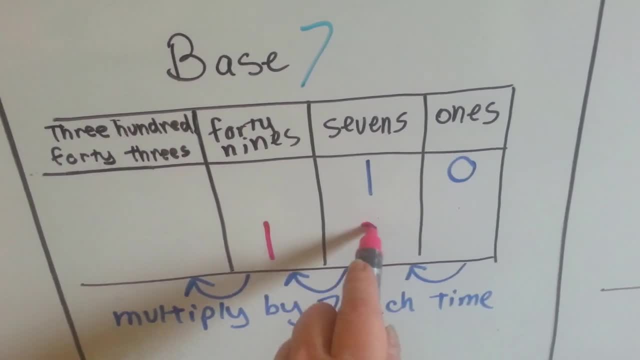 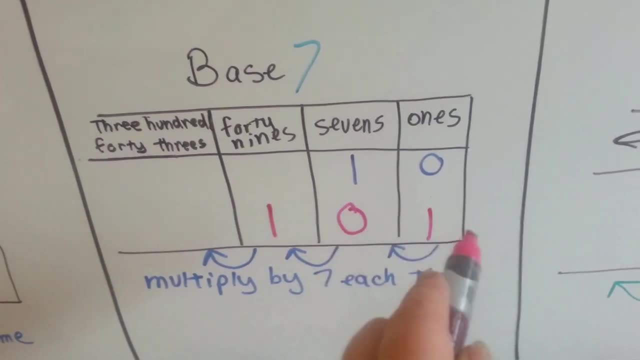 in base 7,, you would have 149,, no 7s and 11.. And that's how you would write the number 50.. A base 10, 50 would be 101 in base 7, because it represents a 49,, no 7s and 11.. Okay, Base. 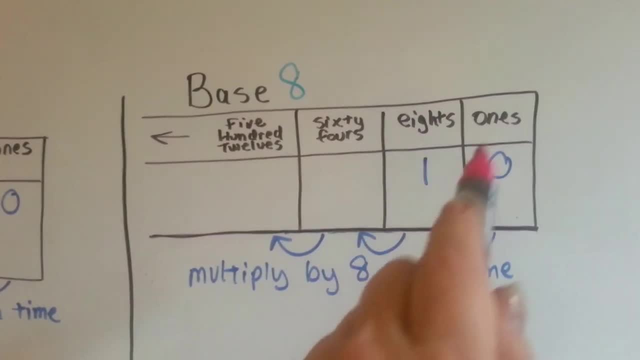 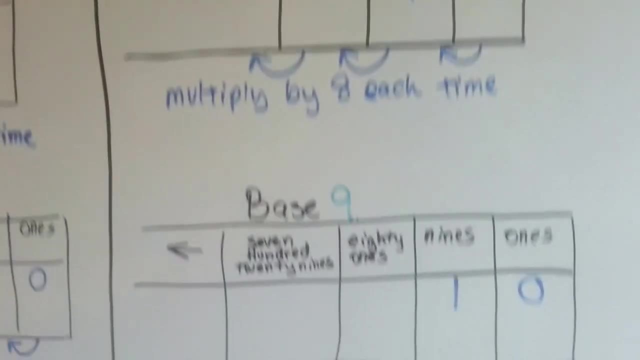 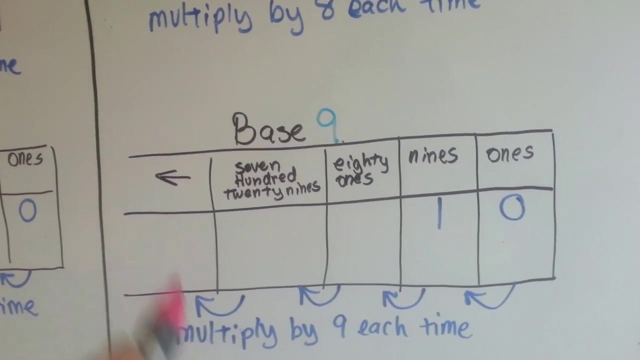 8, same thing. You'd write the number 8 as a 1 and a 0 to represent an 8 and a 0. You 0, multiplying by 8 every time you move over to the new place value Base. 9, same thing. second column is the 9s. you multiply by 9 each time you go over. see. 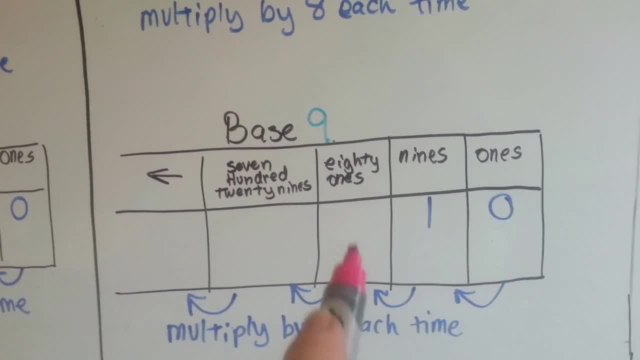 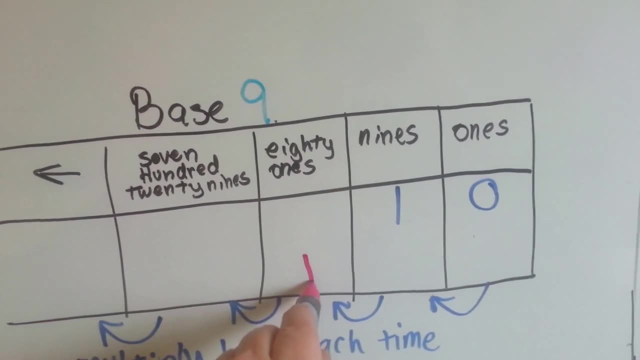 We know it's base 9 because the second column is 9s. 9 times 9 is 81. so here's the 81s column. So if you wanted to write the number 82, you would write an 81, no 9s and 1: 1.. 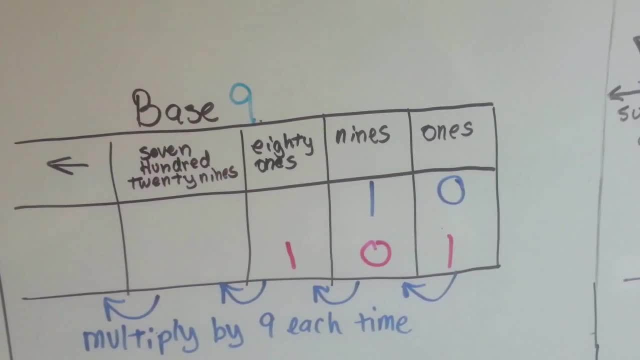 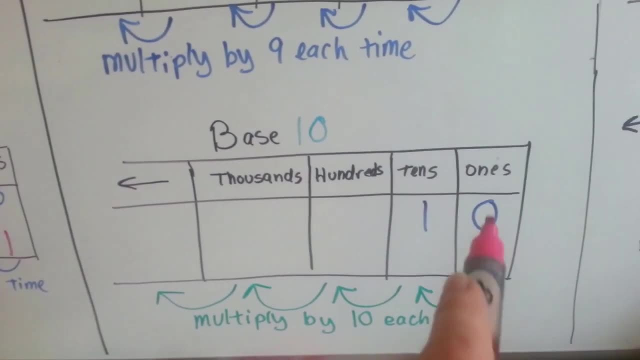 81 plus 1 is 82 in our base 10 system, but 82 in base 9 would be 101, see So in base 10, every time we move to the next column we're multiplying by 10.. 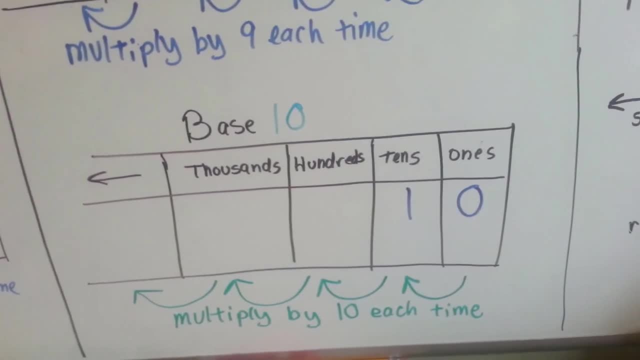 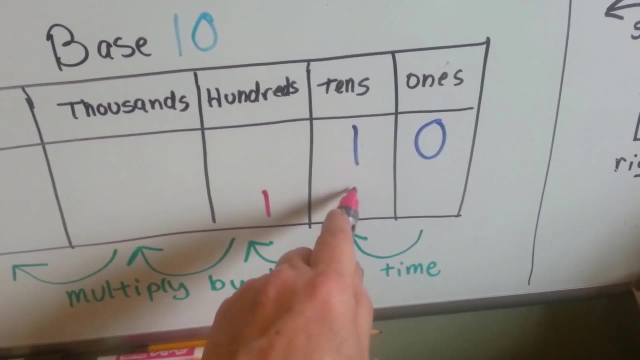 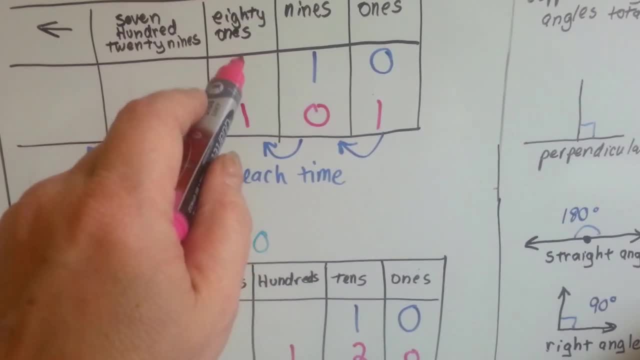 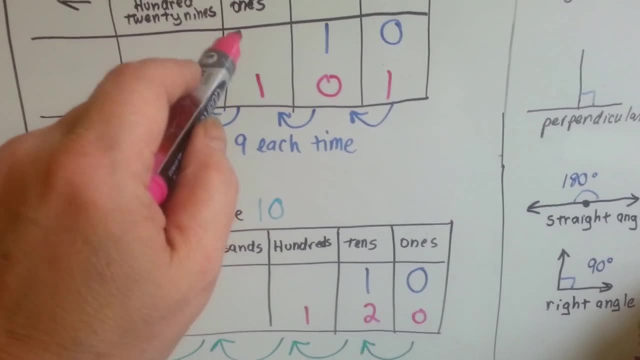 In base 9,, 120, we would write 100, 2 10s and 0, 1s. see be a lot different because 81 times 9 is 729. So we'd have to do several 81s to do it with. 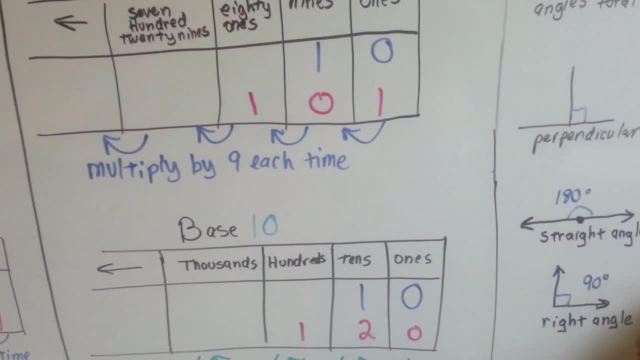 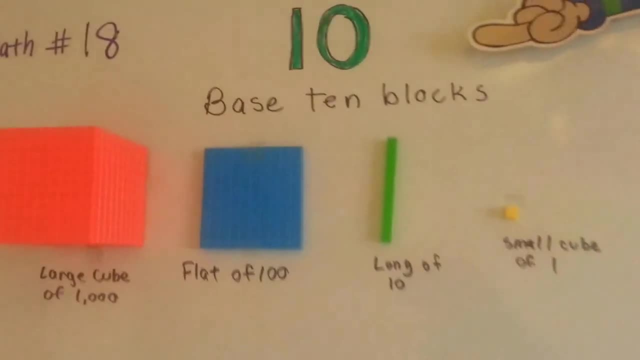 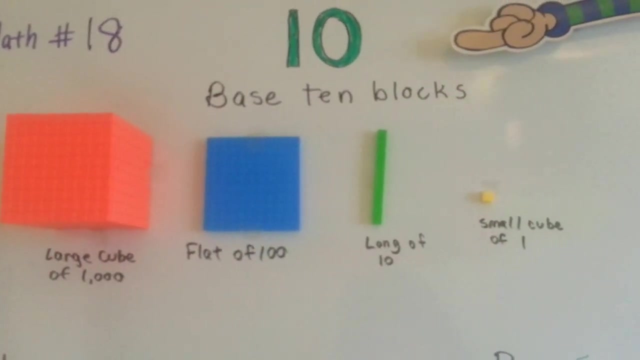 9s and 1s mixed together to make the 120.. See, It would look completely different in the other base systems. So when you think about base 10 blocks, think about how we're multiplying by 10 every time we move to the left. And for those of you that are a little, 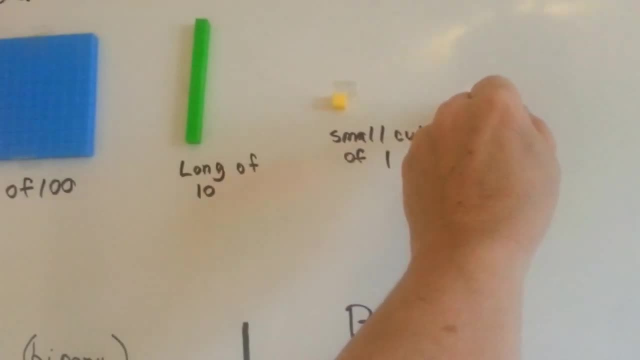 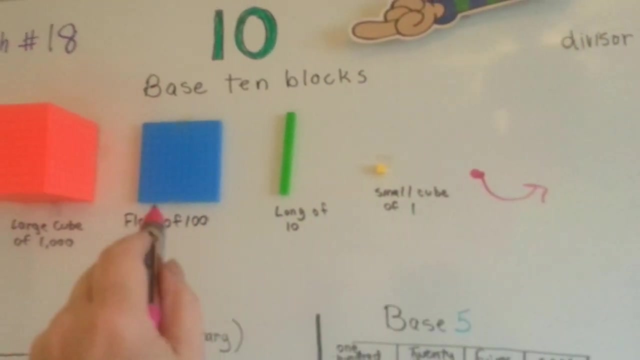 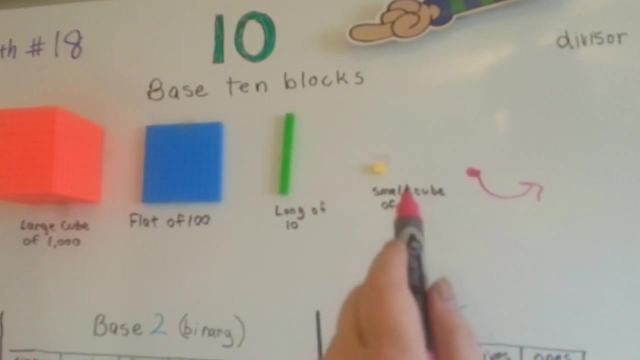 older on this side of the decimal point. we have a decimal point here and as we go this way, we divide by 10.. We're multiplying by 10 to the left and dividing by 10 to the right, because the next place value after 1 is tenths, which is 1 divided by 10.. See: 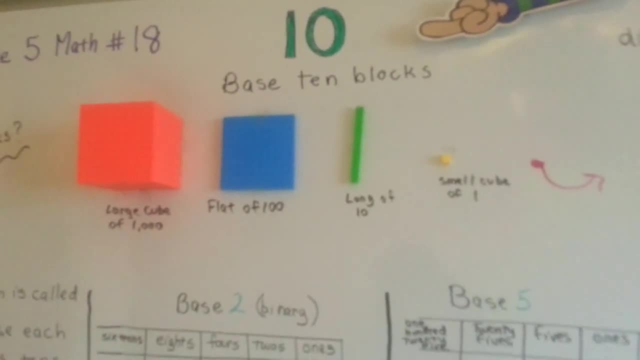 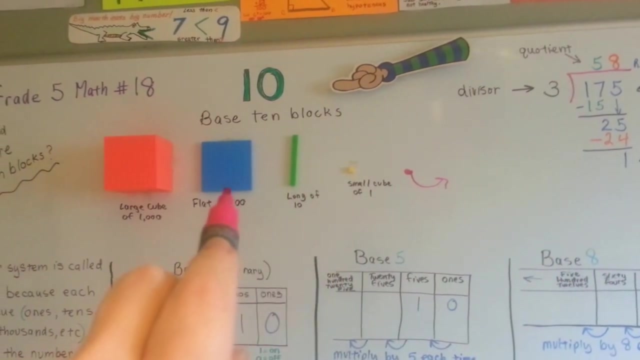 So we're going to divide as we go to the right and we're going to multiply as we go to the left. Okay, That's base 10.. Those are base 10 blocks. You have 1,, then 10,, then 100,, then 1,000, just like our place.